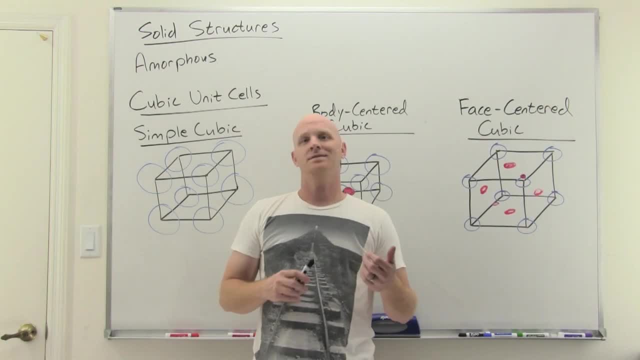 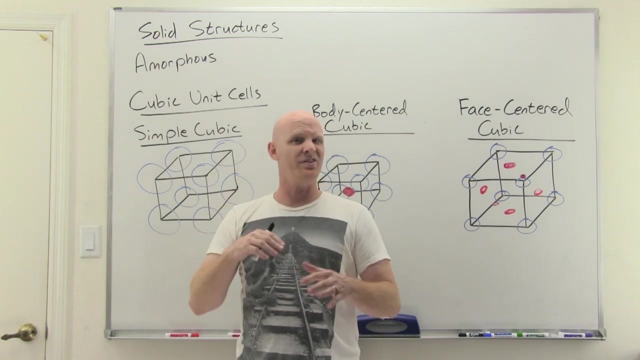 In this lesson on liquids and solids, we're going to take a look at solid structures and we're going to take a look at the different cubic unit: cells: simple cubic, body-centered cubic, face-centered cubic. We'll look at close packing of spheres: hexagonal close packing, cubic close packing. We'll finally finish this off with a discussion of the different types of molecular solids and some real small generalizations we can make about those different types of solids. And, as always, if you learned something from this video like it, share it and subscribe if you'd like to be notified when I release more of these. 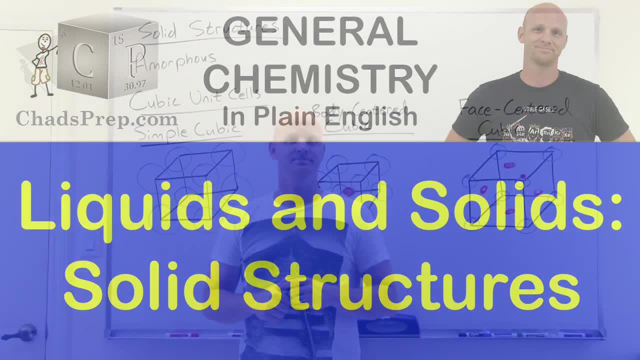 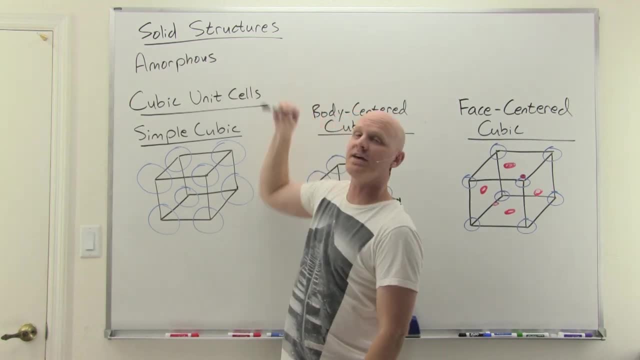 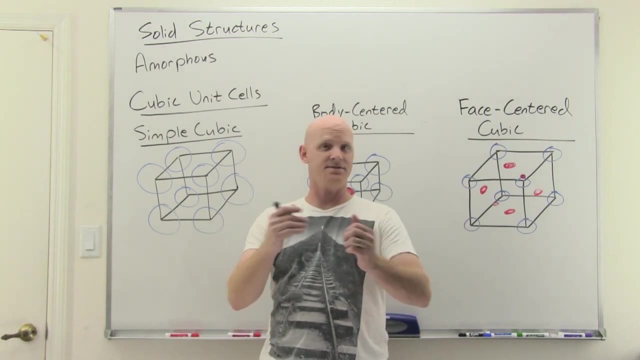 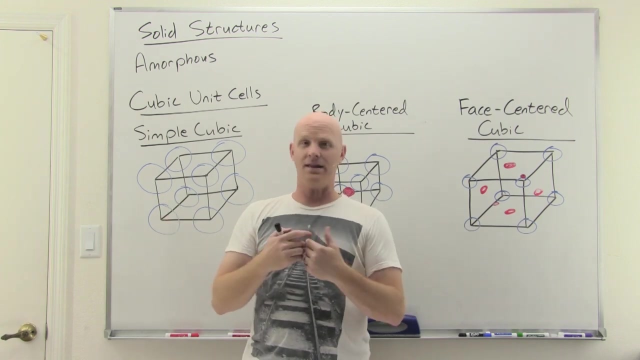 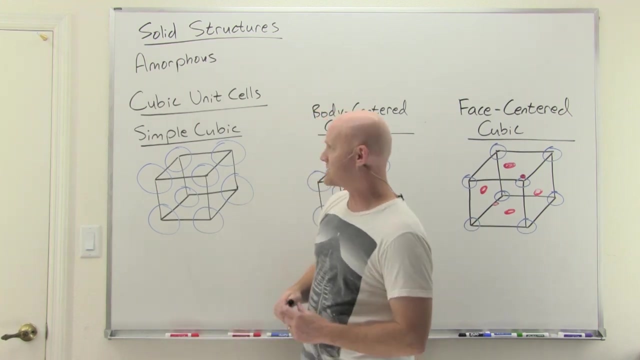 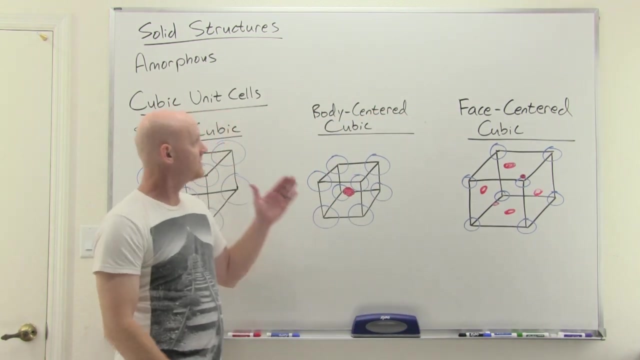 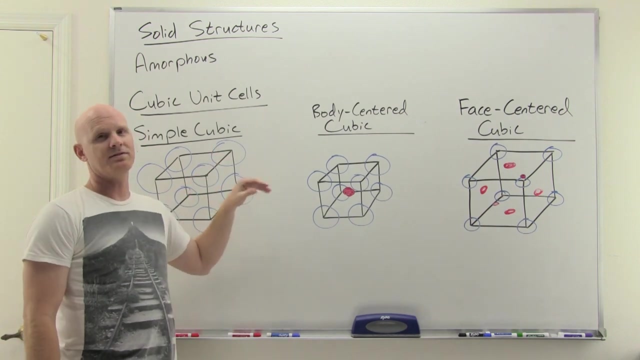 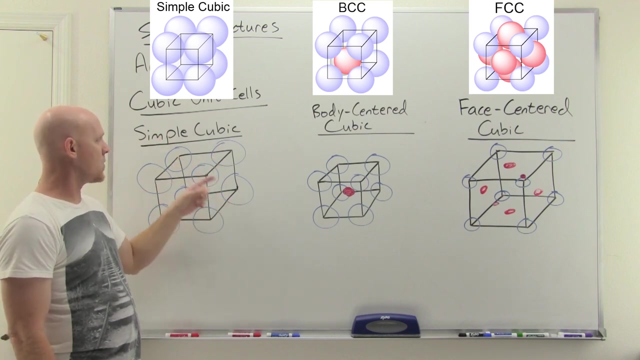 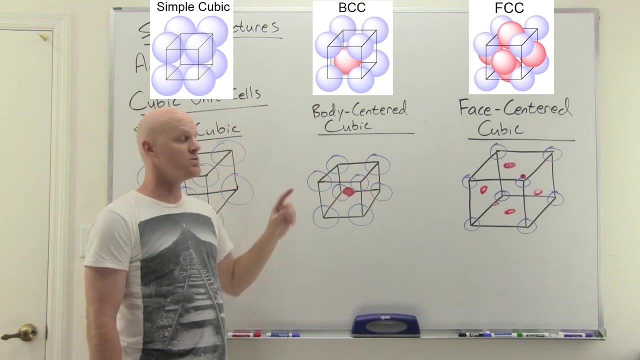 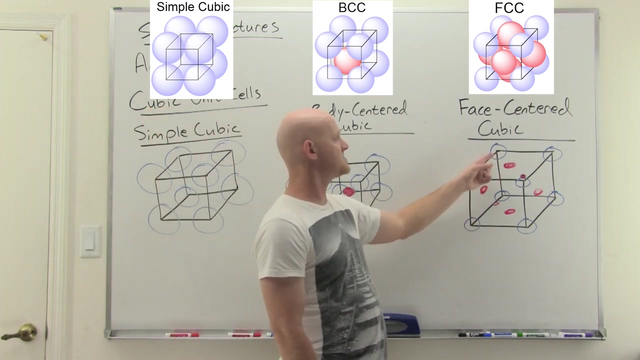 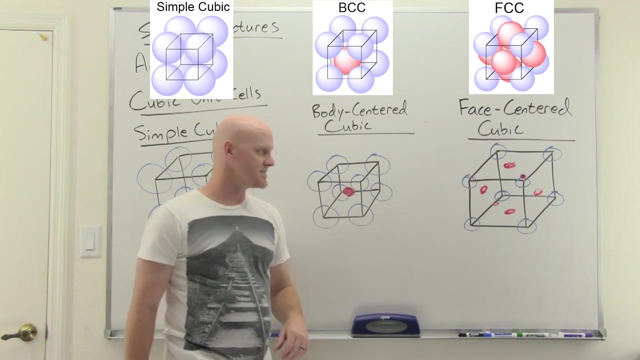 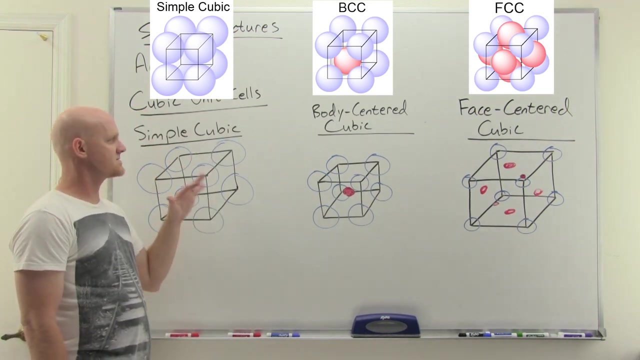 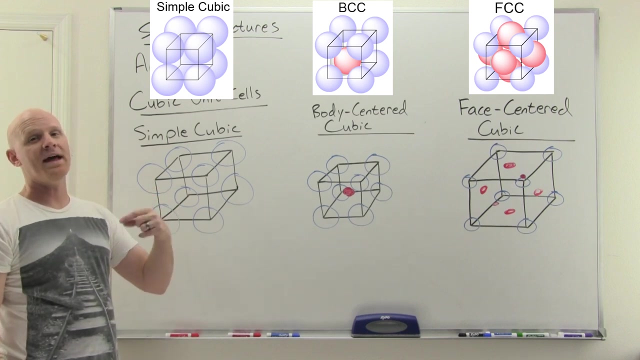 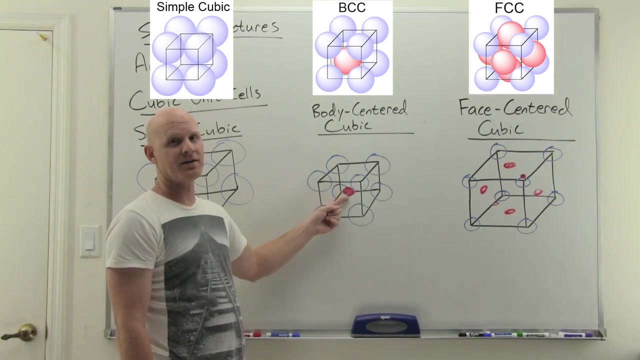 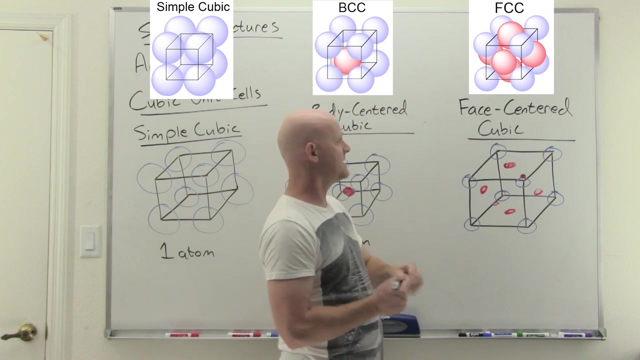 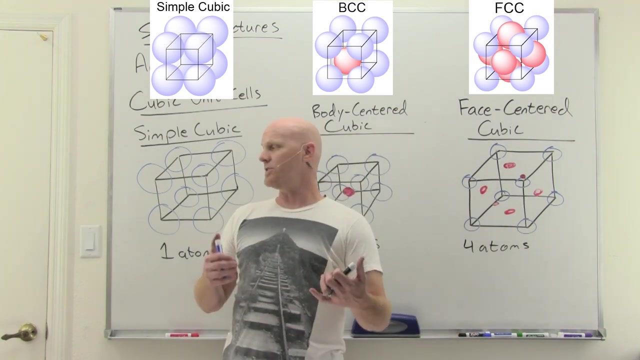 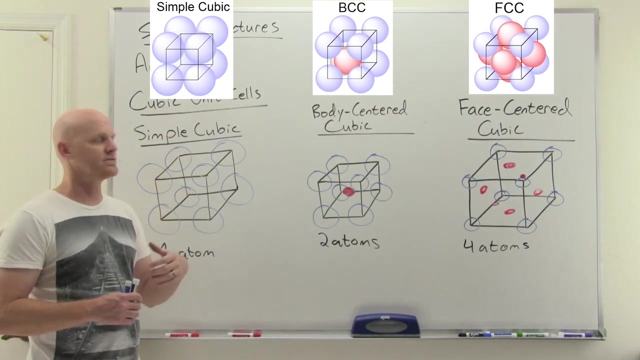 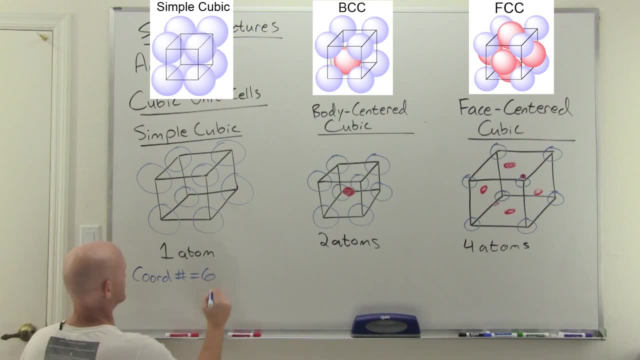 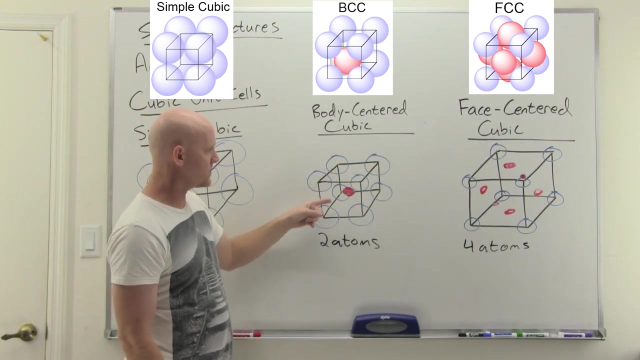 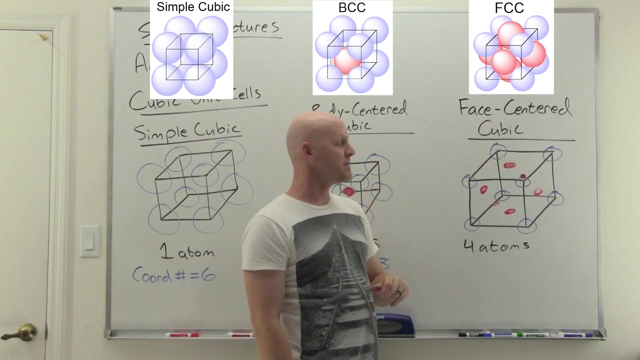 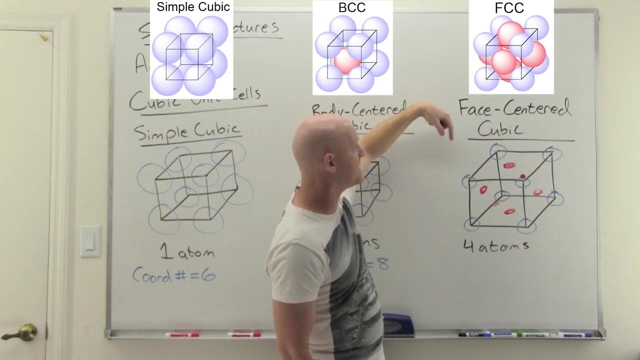 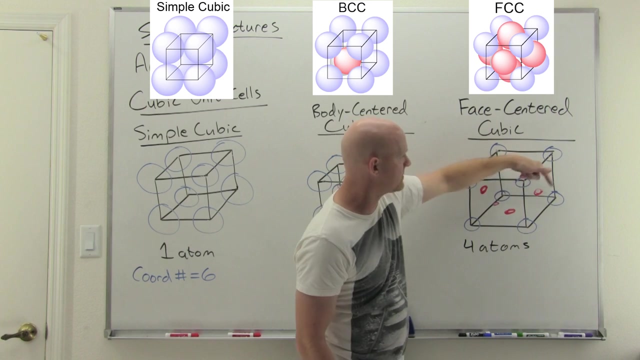 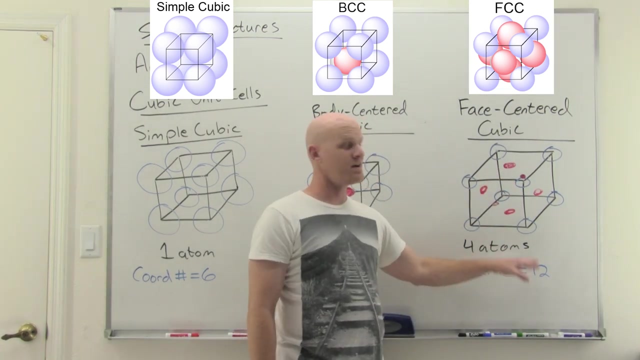 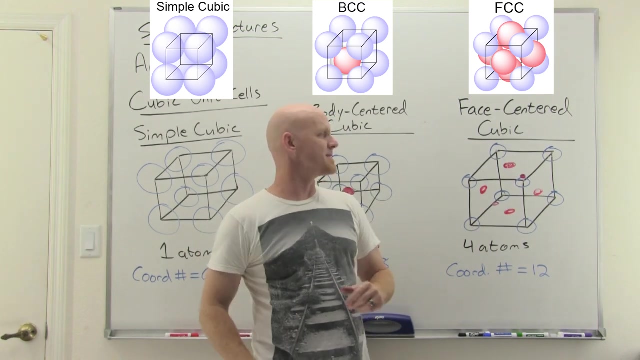 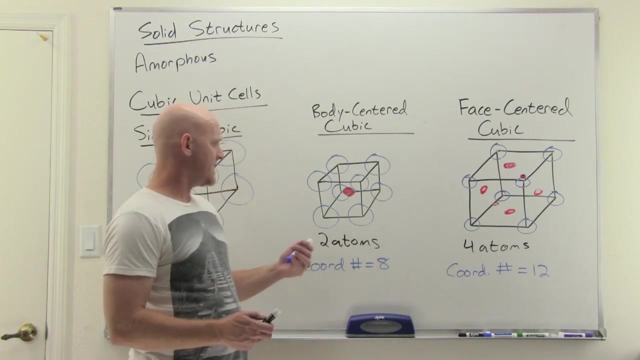 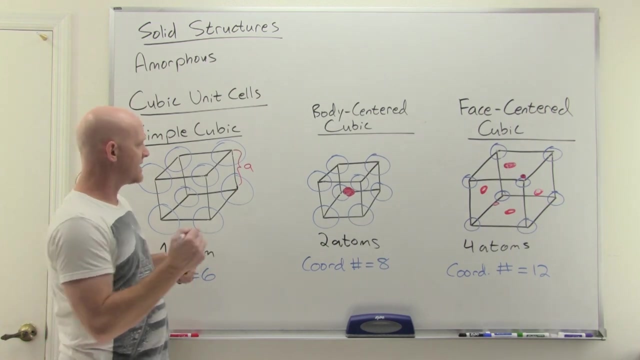 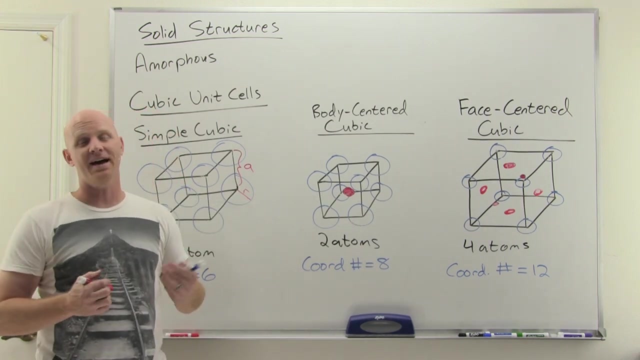 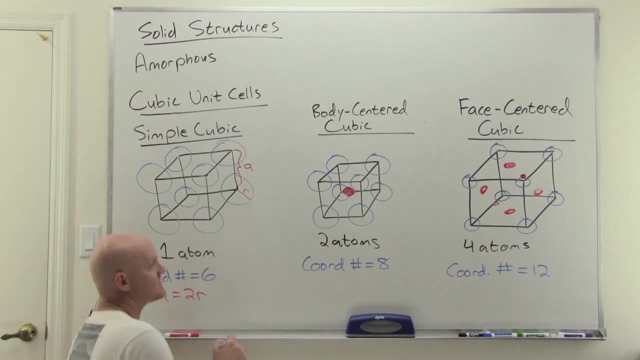 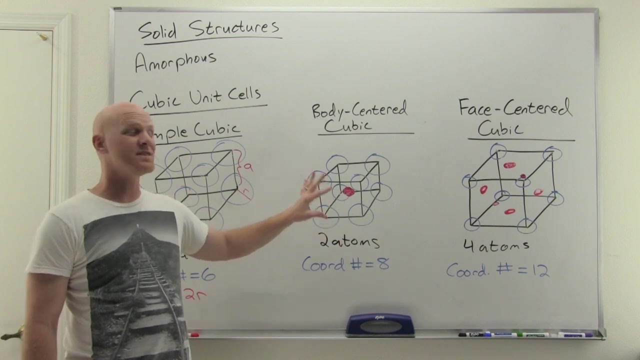 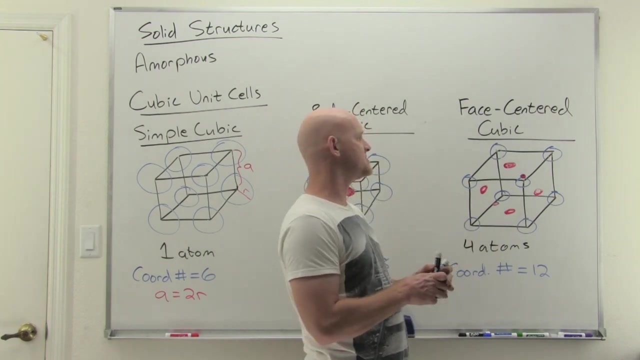 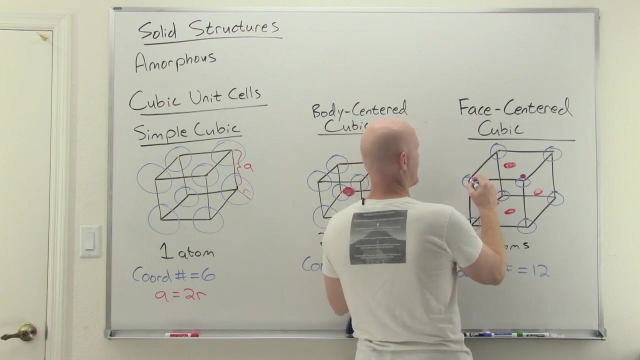 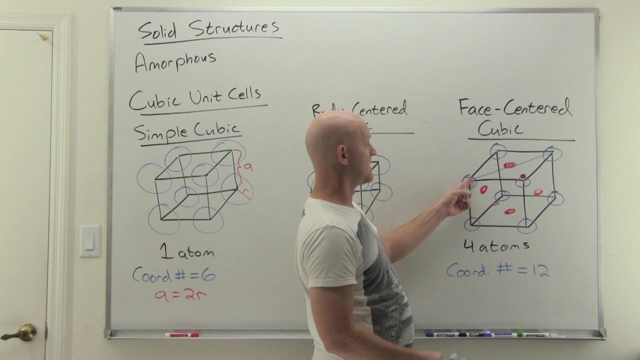 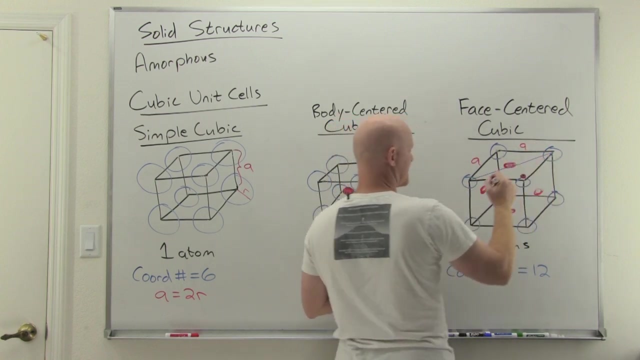 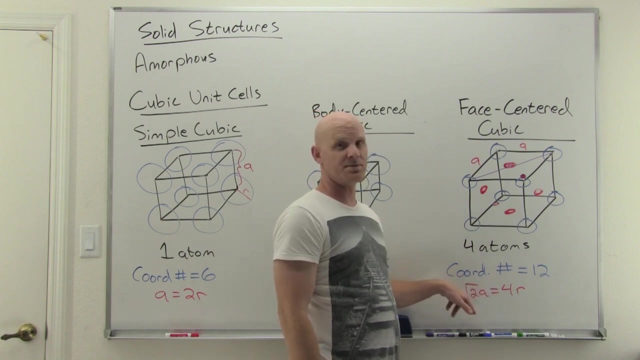 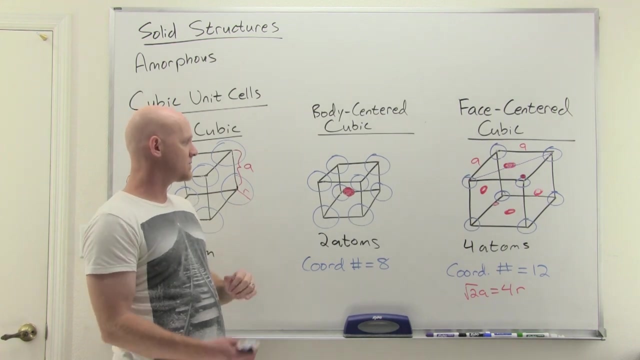 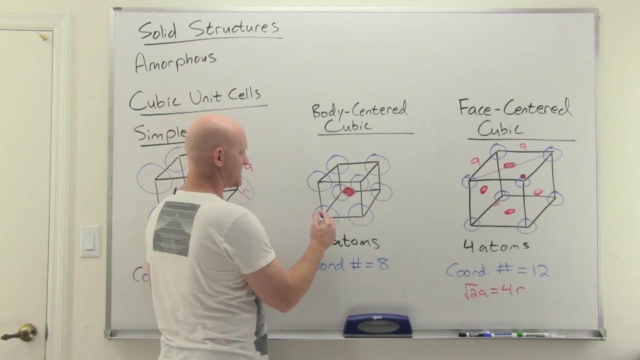 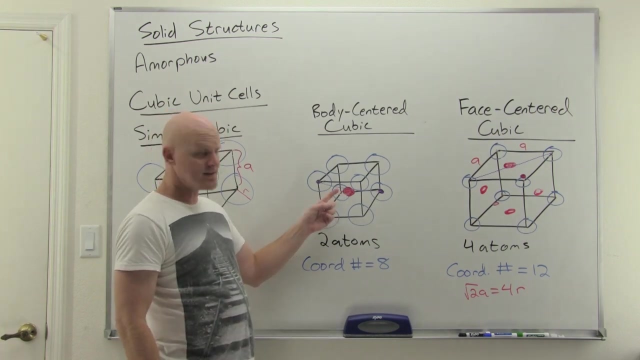 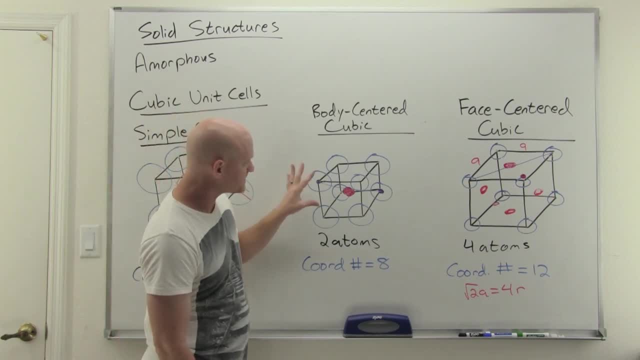 I'll see you next week. Bye, Bye, Bye, Bye. here they were. so in this case, then, it's that body diagonal, and that body diagonal is going to be hard to see. so what we're going to do is draw this triangle right here with a right. 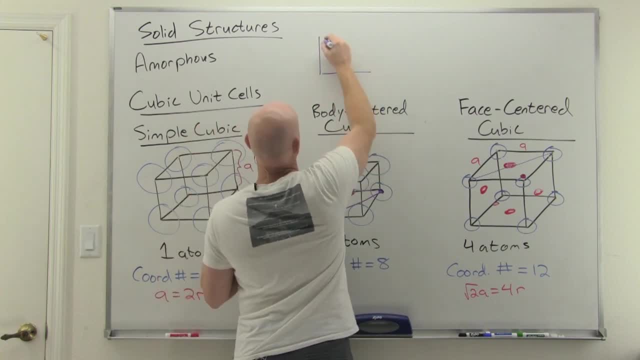 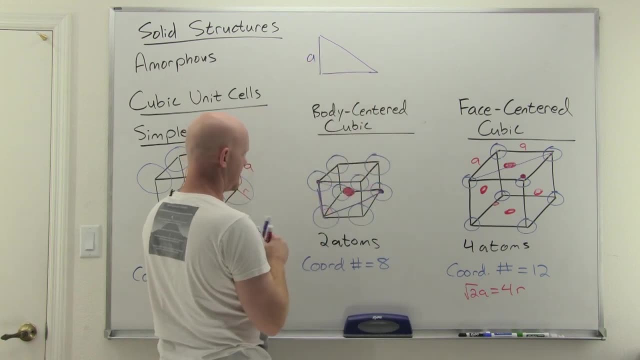 angle right there. so let's draw that triangle, we'll pull it out, and so in this case, this is the edge length again, just simply a here. this is the diagonal across one of the faces, which we just a second ago learned is the square root of 2a, and if you work that out, 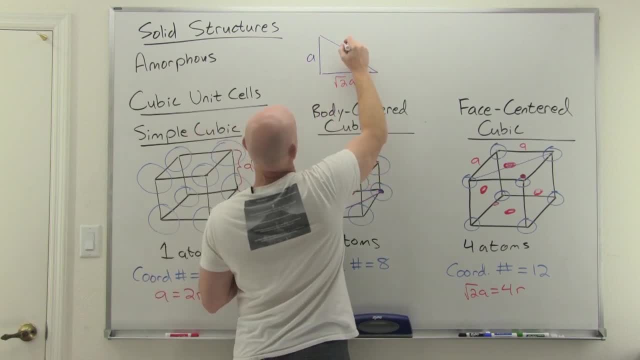 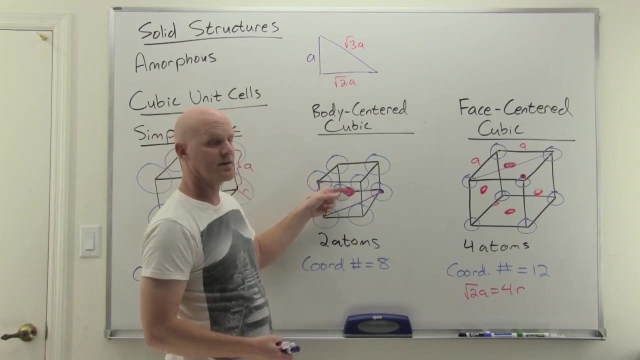 then pythagorean theorem: a squared plus b squared equals c squared. this comes out to equal the square root of 3a. so, and that square root of 3a, right across the body diagonal, again entailed, comprised of four radiuses, and so we get our last relationship here. 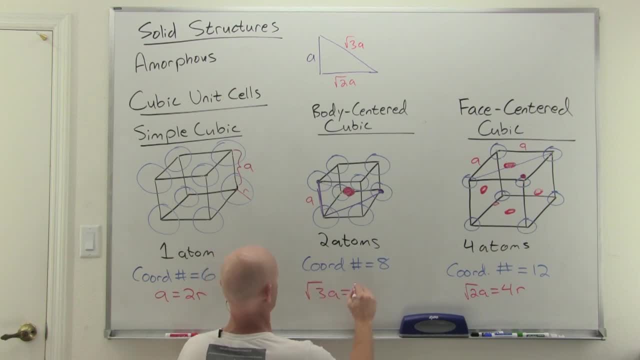 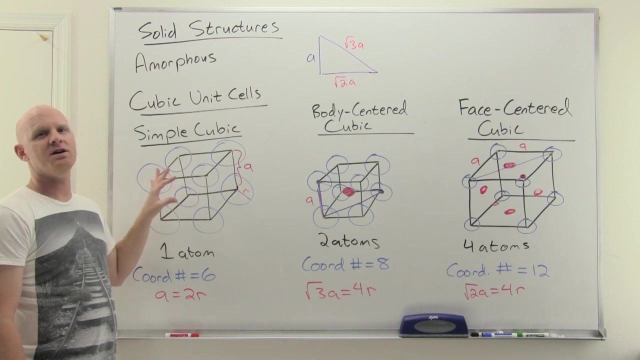 so, Mhm, the packing efficiency of just a measure of the entire volume of the cube. what fraction of that volume is actually atoms relative to empty space. so, like in terms of simple cubic area, you have to know that the volume of a cube is a side length cube. so in this, 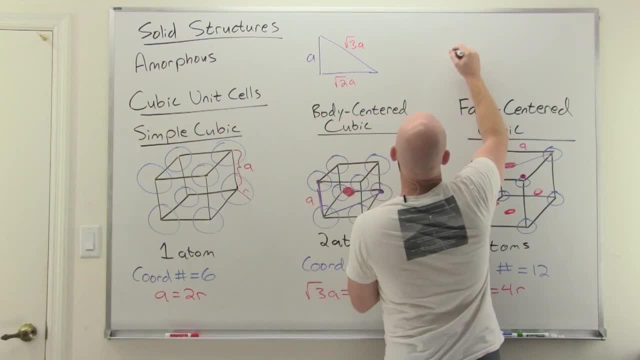 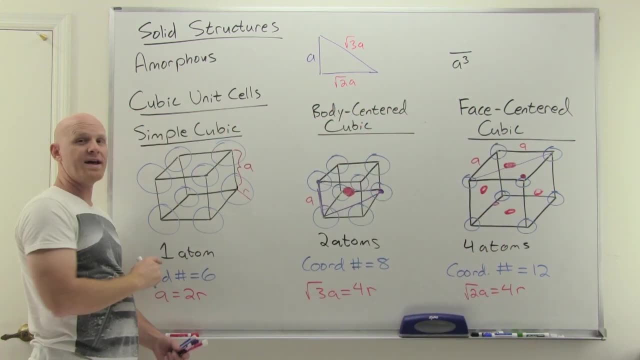 case a cubed, and so packing efficiency is the volume x a mass of v square minus one. efficiency is always going to be over a cubed. So in a simple cubic you have a total of, again, an occupancy of one atom per unit cell. Well, you're supposed to know that atoms are spherical. 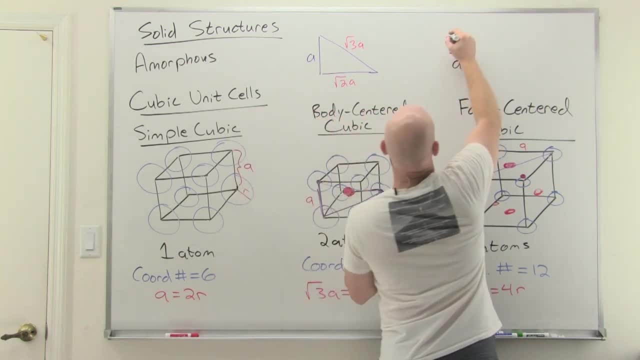 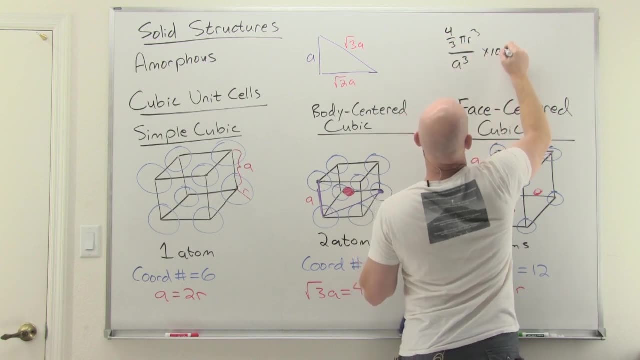 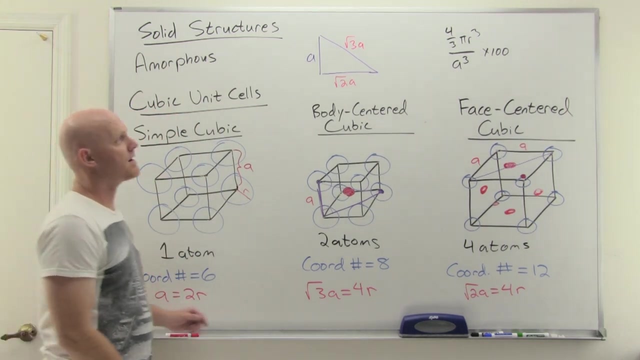 and the volume of a sphere is four thirds pi r cubed, And so here we'd have four thirds pi r cubed over a cubed times 100.. And that would be our formula for the simple cubic. And we just have to take into account that a equals two r, And so we could replace a with two r, or we could. 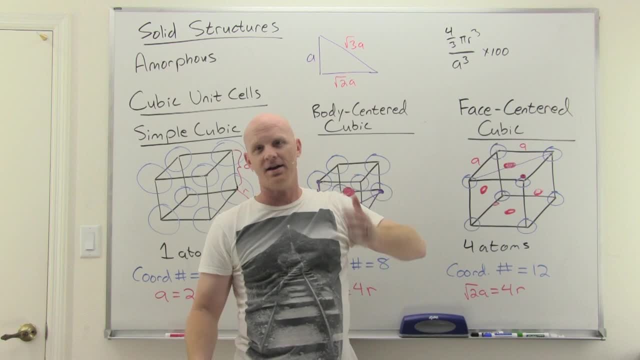 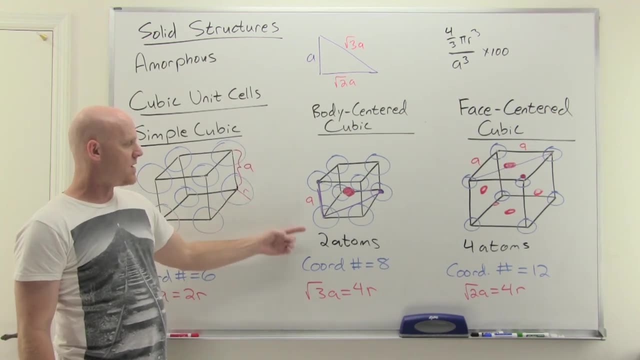 replace r with one half a, So to make this work out and have the a's or the r's, cancel and stuff like that. But the math would work out great. It would be similar here, with the body centered cubic, except now we have two atoms per unit cell And so the volume of the atoms wouldn't be just. 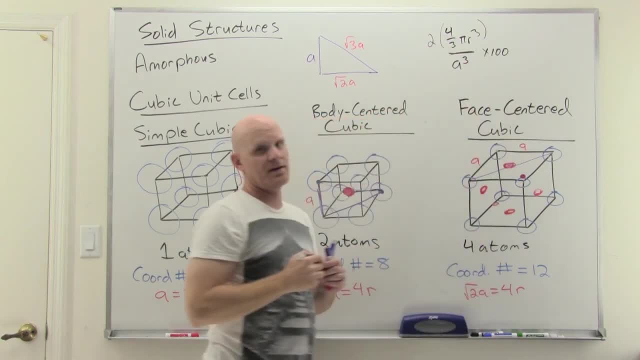 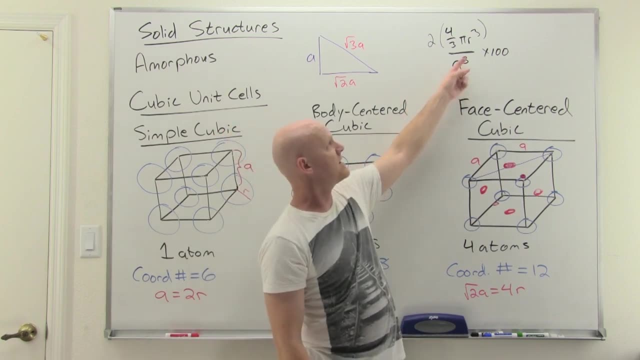 one sphere, it would be two spheres. So, and now also our relationship between a and r is different. And again, we could solve for a and subsequently it in right there and get the r's to cancel. or we could solve for r and substitute it right in. 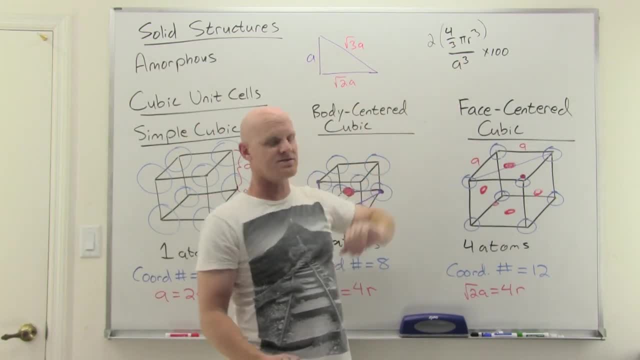 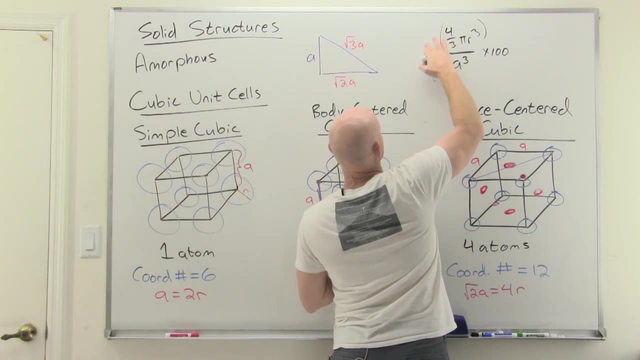 there and get the a's to cancel. Either way though, we could calculate a packing efficiency, And finally we'd get a similar equation if we did this for the face centered cubic, But instead we have four atoms per unit cell, And so the volume of the atoms would be four times four. 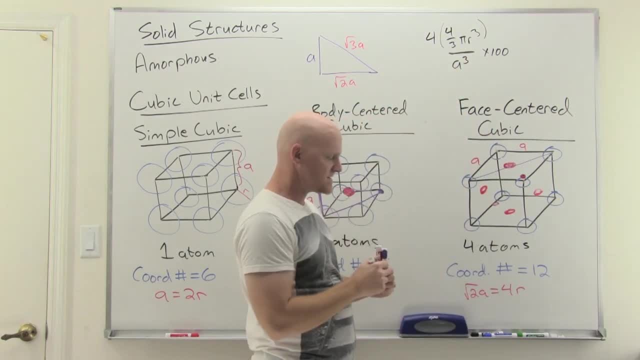 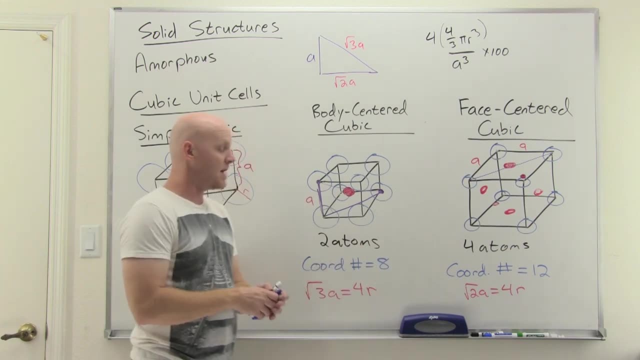 thirds pi r cubed divided by the entire volume of the unit cell, And once again we'd have a, now an even different relationship between a and r and have to make a substitution one for the other to get this to work out. But when you actually take the time to do this, 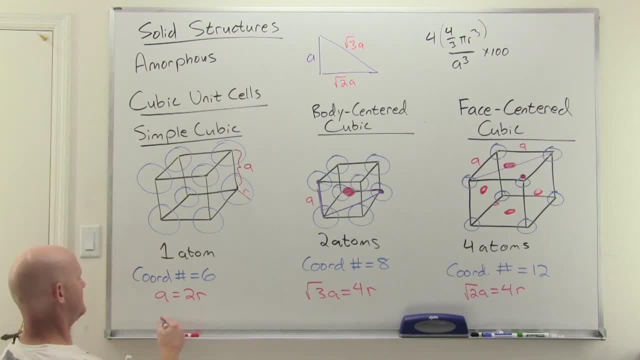 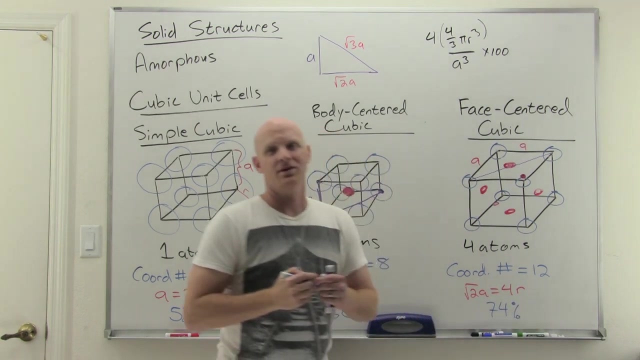 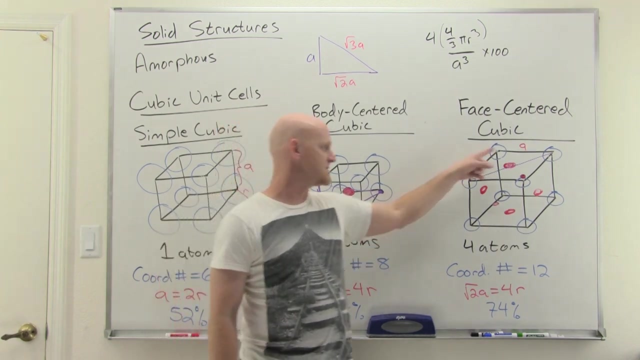 so if you got your study guide in front of you, you can see that you go from 52% here packing efficiency, to 68% for the body centered cubic, up to a maximum here of 74% for the face centered cubic. So, and you don't have to know those numbers, but you should have in your mind, though, that the face centered cubic has the greatest packing efficiency, has the least amount of empty space inside. That's something worth memorizing, but the numbers themselves not super important. 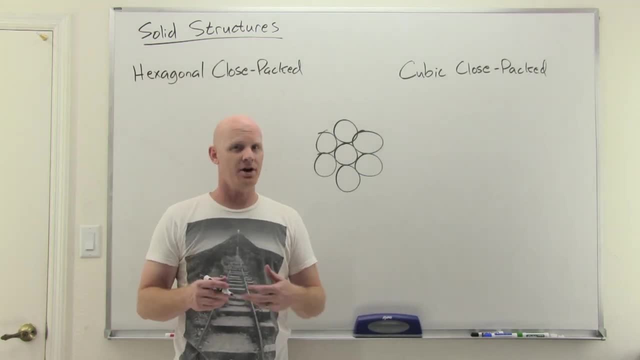 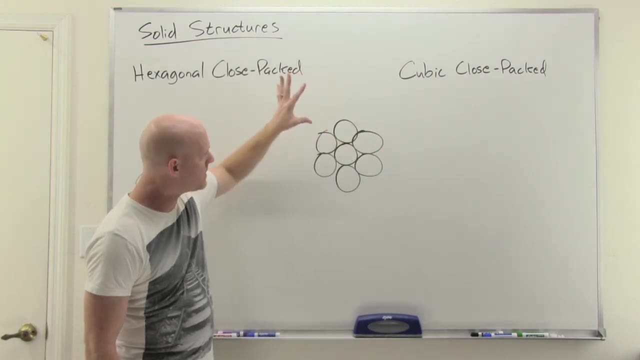 All right now. we got to spend a little bit time talking about what's called the close packing of spheres, like a couple other different solid state structures, And there's two types here: hexagonal close packed and cubic close packed, and they're all based on this kind of base structure. 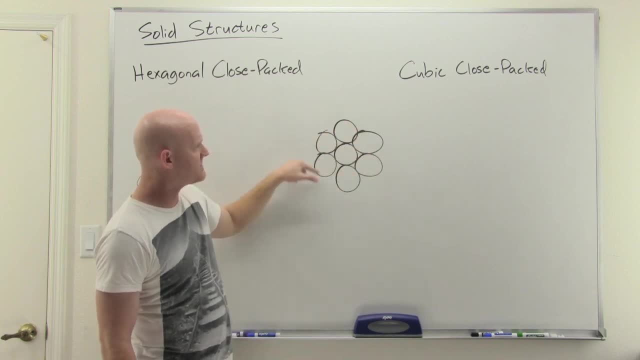 So you've got a layer of atoms here, and there's one in the center, And, for all the same size spheres, you can fit exactly six right around it, So, and that would constitute a layer. So what you find, though, is that, if you actually picture these as spheres, 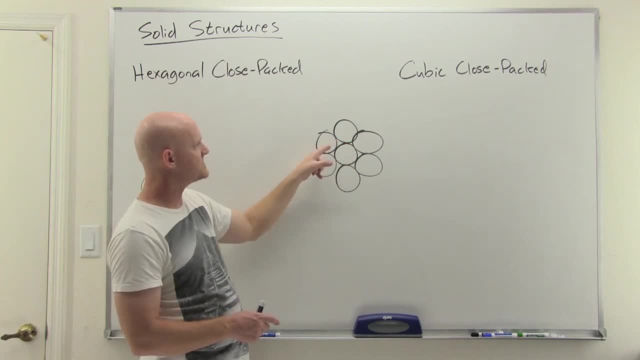 and you lay it down flat- is there'd be small little indentations where you could fit layer of atoms on top and they would rest right into those little recesses to kind of maximize the space being used. and so if we look at kind of the next: 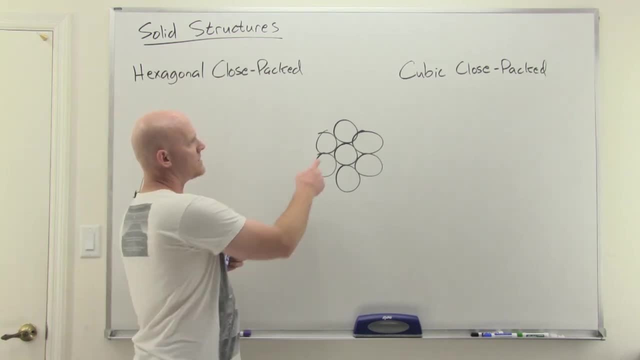 layer. here you've got your choice on where the next set of balls could like kind of rest in place and stuff like that. so if we take a look and say maybe we rest one of the next layer right here, well, because I've used that spot right. 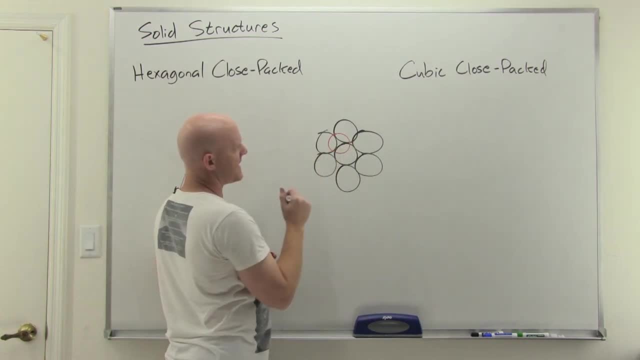 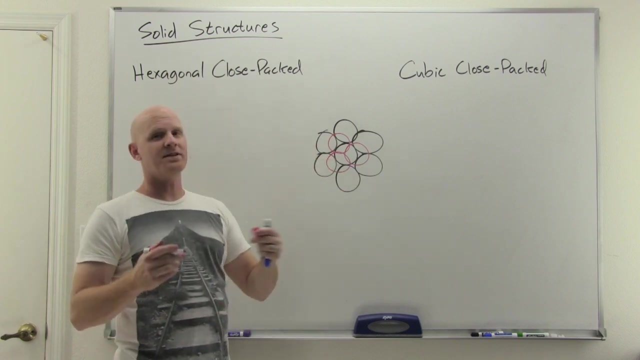 there. that automatically rules out that I can't use that spot or that spot. so but I can use this one and this one. it turns out just like so cool and I could make another one of these six around this center atom or something like that along the way. so but you get this other layer and it turns out I didn't again. 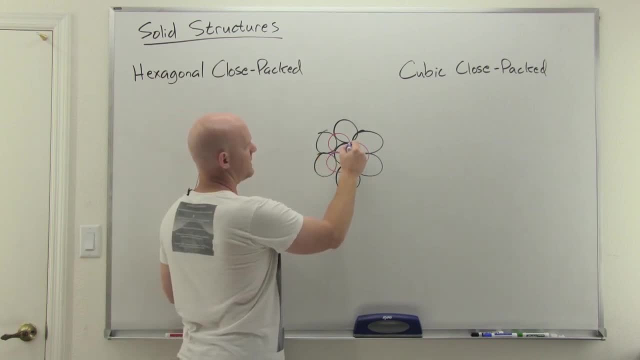 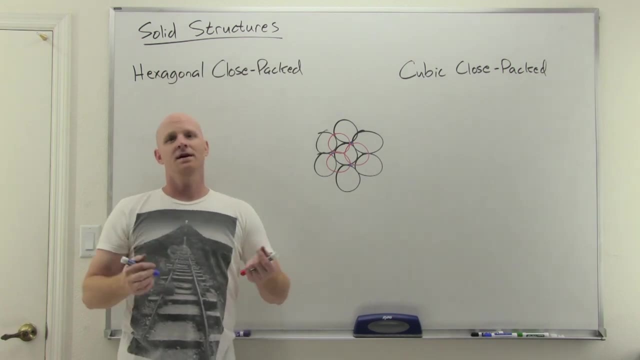 get to use this hole right here, or this hole right here, so, or this hole right here, it turned out, so we didn't get to use those on this one. now I've got this first layer in black, the second layer in red, and again we're limited by 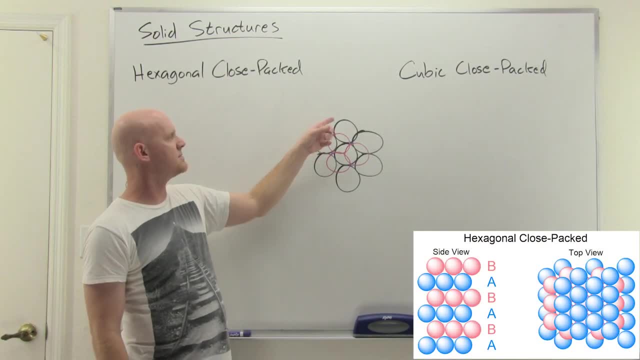 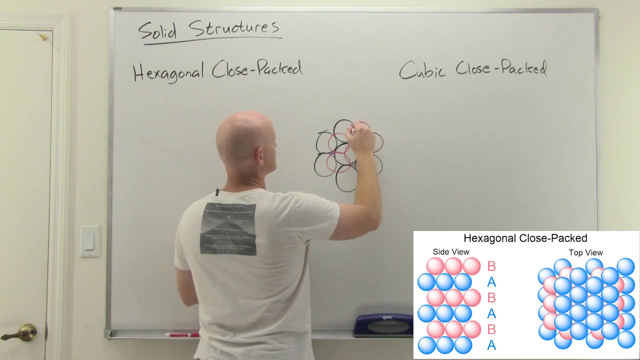 my artistic ability here. so. but if you just repeat the black layer over again- and maybe I should draw a few more of these on here just for the fun of it, so get a full red layer on there. so but if we just repeat the black layer in the 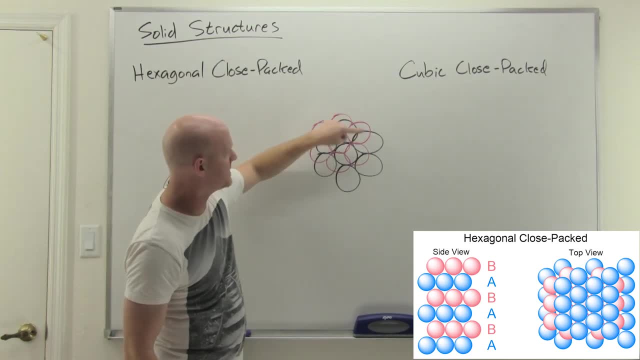 next layer, out further so and just write where the black ones are, put another set of balls on top. so if you just repeat the black layer in the next layer, out further so and just write where the black ones are, put another set of balls of black ones, and just have an alternating, repeating pattern of two layers, that's what. 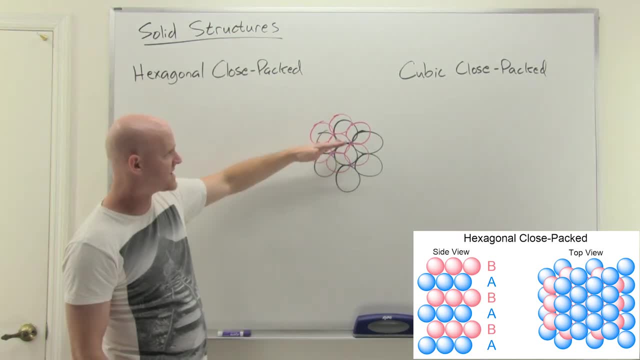 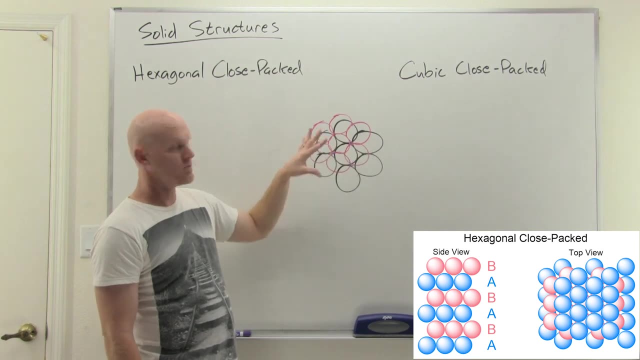 hexagonal, close-packed, looks like It's just alternating two layers and if you turn this sideways, we like to just say it's A, B, A, B, A, B, where every other layer is in exactly the same relative lattice positions as two layers before it. All right, cubic, close-packed on the other. 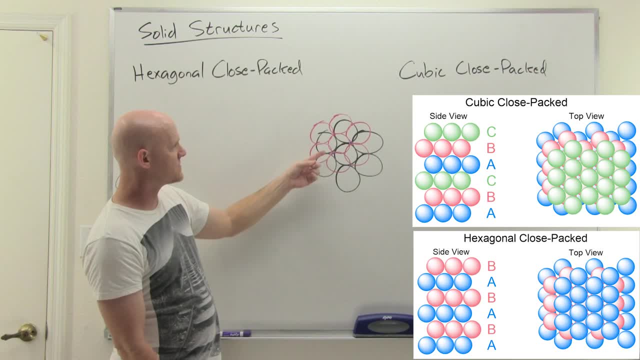 hand has an alternating set of three layers, because the ones we never used notice that hole right there is not only a hole where it was for the black layers and we didn't use it, but it's also a hole in between these three red ones right here as well, and so this next layer has a choice. 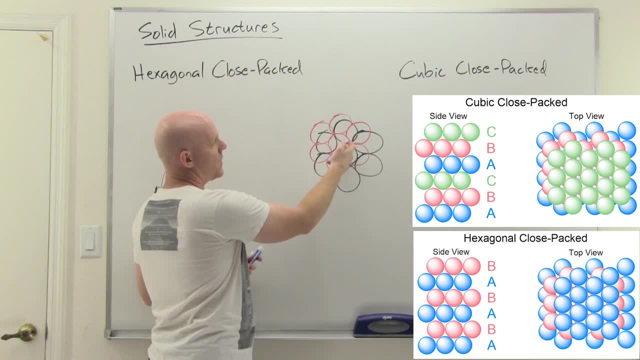 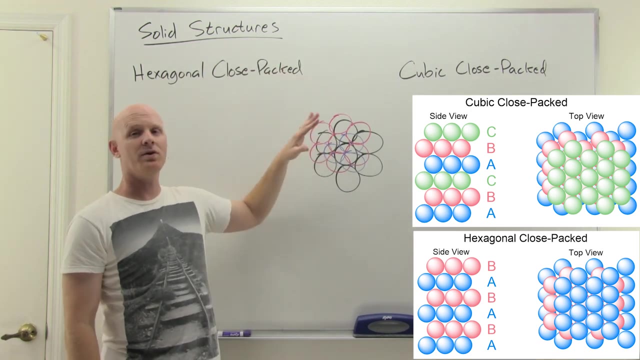 It can go back and repeat the holes where the black ones were, or it can use the holes we've never used here instead, Cool, and then I could have this third layer so as well, and then go back and repeat the black layer and then the red layer, and then the black layer, and then the. 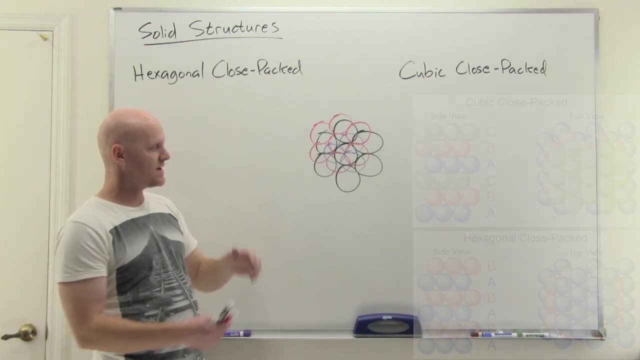 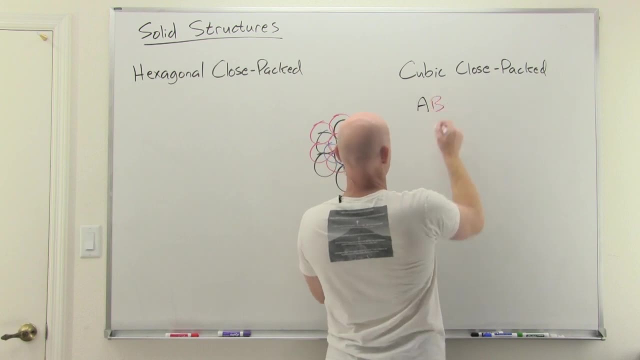 blue layer and work this out further and further and further, and so here we'd have this repeating three-layer and we like to say A, B and C repeating each other, and then again A, B and C, yet again, so something along those lines. We're again back over here with the hexagonal. 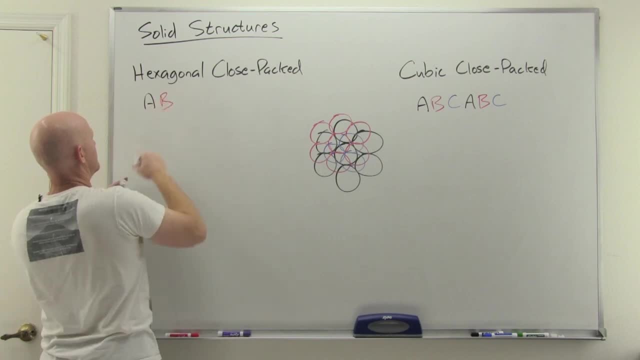 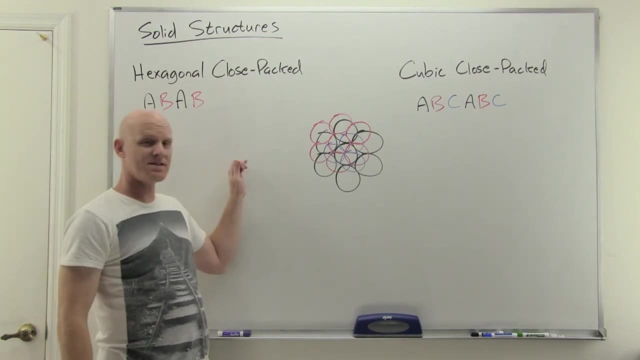 close-packed, It's just A and then B, and then A and then B, and just the same thing, The two repeating layers, and that's the big difference. Now, it turns out, both these have really high packing efficiencies. They both have coordination numbers of 12, so, but the big thing, 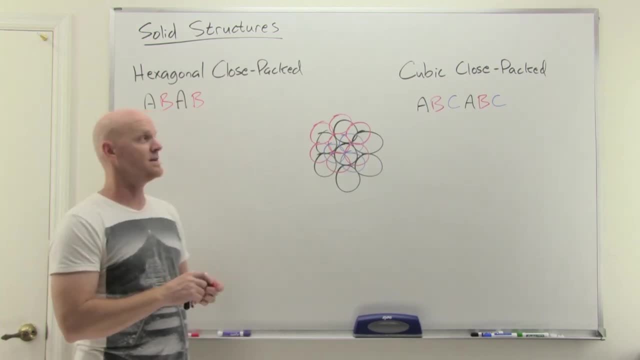 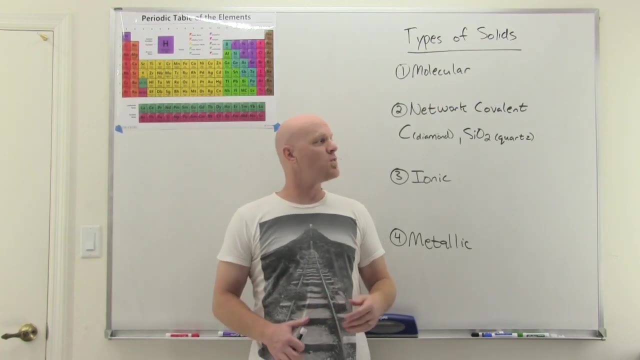 that usually you might be expected to know is just the pattern. Is it a pattern of two repeating layers or a pattern of three repeating layers? All right, last thing, I just want to compare the four major types of solids, so many. we've already talked about A couple. we want to specify a couple. 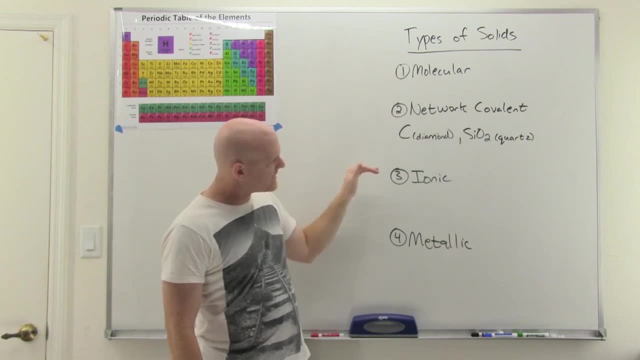 more things about so, but there are molecular solids, network covalent solids. I don't know if you're familiar with ionic solids, metallic solids and your molecular and network covalent composed of all non-metals, your ionic metals with non-metals and then metallic all-metals. 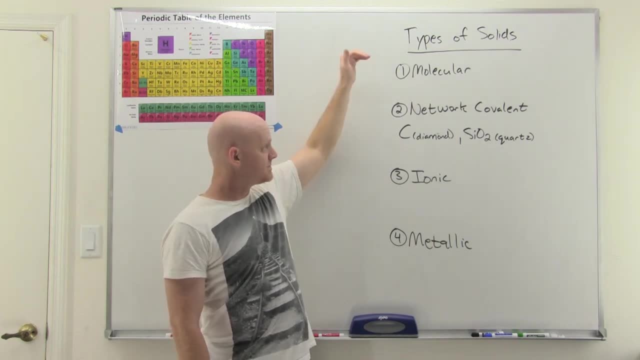 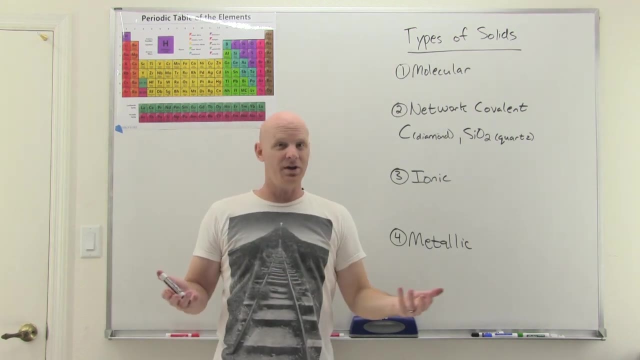 If you look at your molecular and network covalent. so by far, when you've got non-metals, by far the vast majority are going to be molecular and what holds a molecular solid together is just, you know, intermolecular forces, hydrogen bonding, dipole-dipole forces. 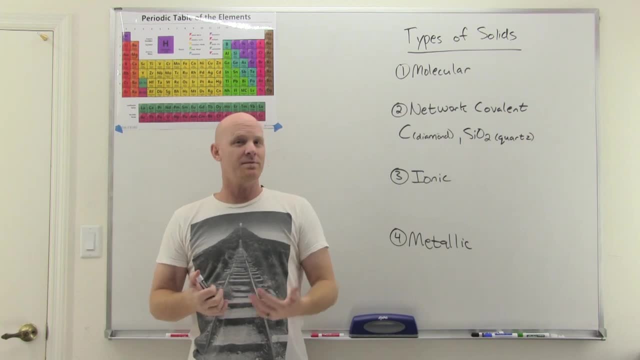 London dispersion forces which are rather weak when you compare them to the strength of a covalent or ionic bond. so network covalent solids are held together by covalent bonds, Ionic compounds are held together by ionic bonds and the vast majority of both the network. 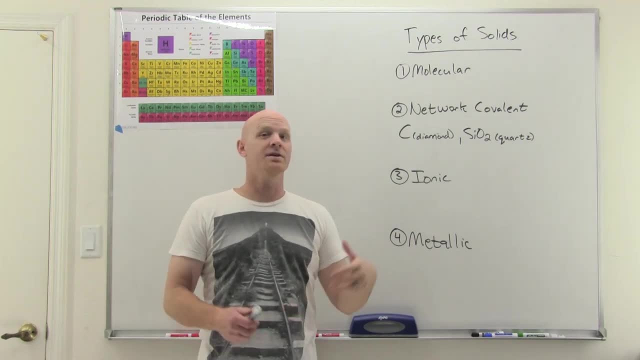 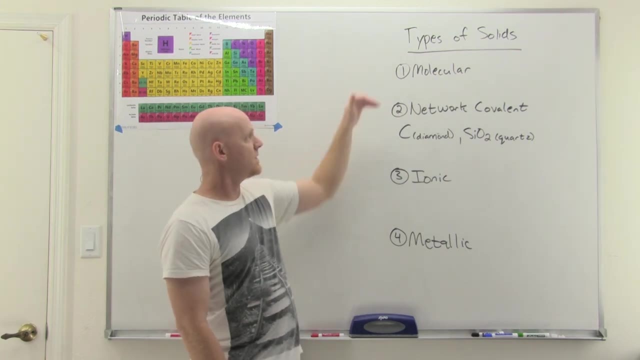 covalent solids and the ionic compounds are solids at room temperature, so to melt them you actually have to break bonds, and that's really difficult, and so at room temperature you don't have enough energy to break those. so whereas most molecular compounds, you know, 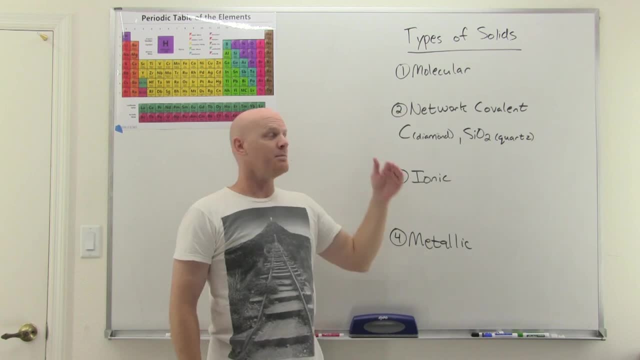 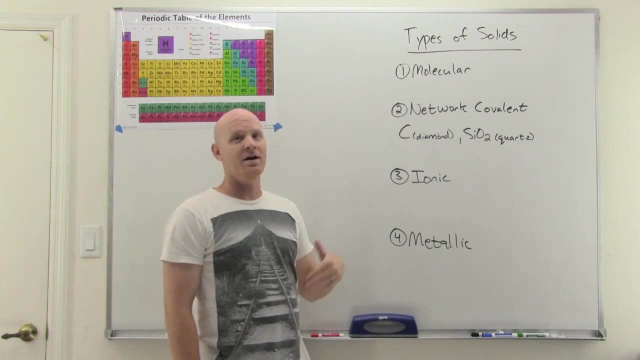 we can find them in solid, liquid and gaseous phases, depending on size, but generally, if you're going to find something existing as a liquid or a gas at room temperature, it's probably going to end up being a molecular compound. There'll be a few exceptions, like we've 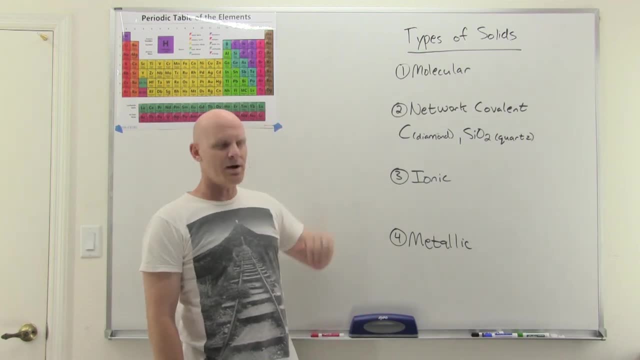 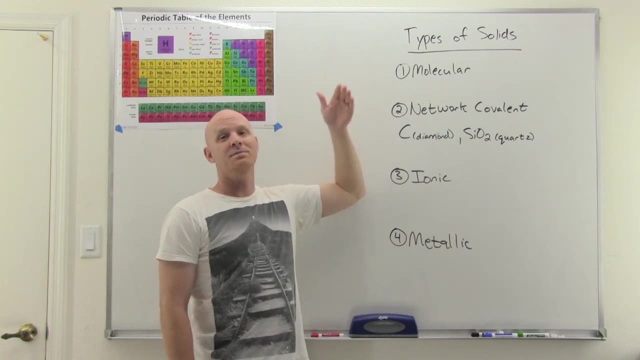 got, you know, mercury metal so, and a couple of metals that are just above room temperature might melt, and stuff like that. However, the vast majority again, of compounds that are liquids or gases at room temp, they're molecular compounds because the forces holding them together are. 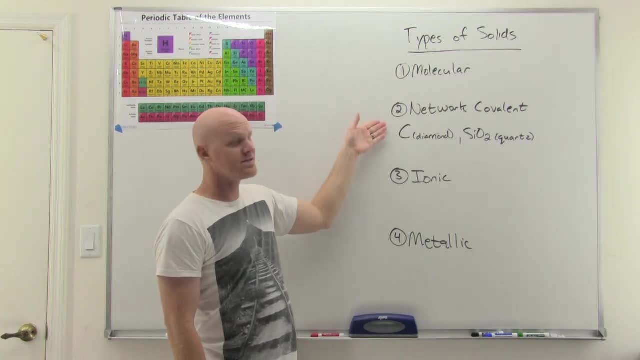 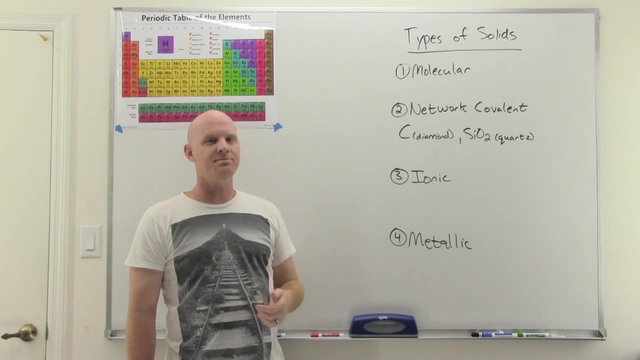 rather weak in comparison to the rest of these Now network covalent solids. there's just a couple examples here and we covered that back in chapter eight. so you got diamond quartz and maybe even they'll throw graphite, another form of pure carbon, on there and things of that. 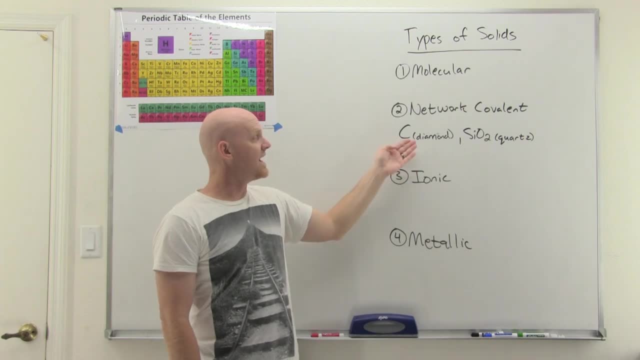 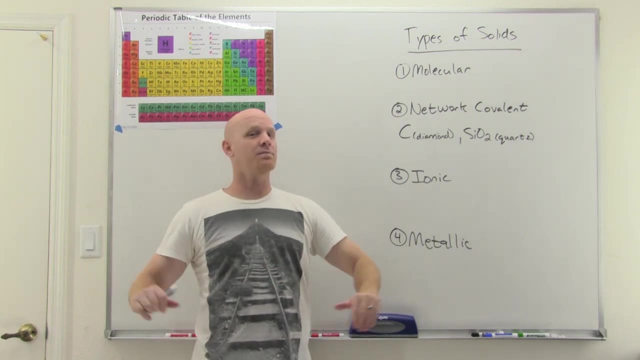 sort and they're held together by covalent bonds. so, and you might just know that diamond's crystal structure has all of the carbon atoms in a nice tetrahedral lattice, and suffice to say you probably know as much as you need to know about the crystal structures of these network covalent 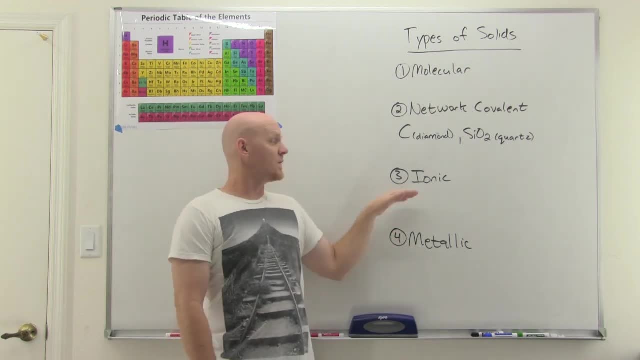 compounds. Now for ionic compounds. you can kind of run away with this if you want to. so, and if you go to a little more of an advanced inorganic class, you probably will and you'll start talking about some of the different crystal structures and the zinc blend structure and the cesium. 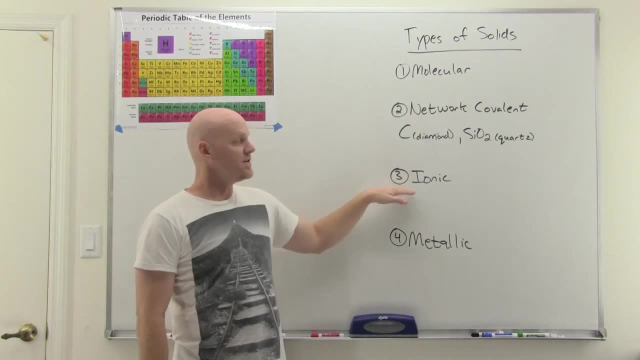 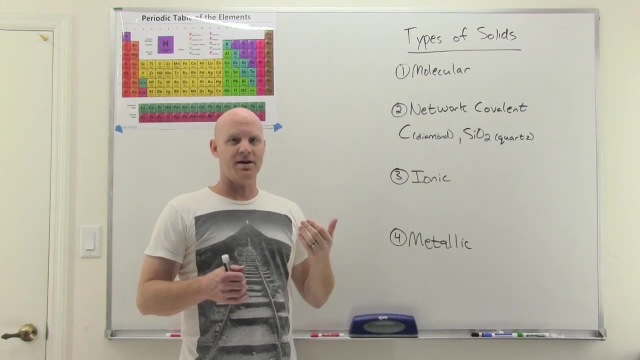 chloride structure, and I'm not going to get into that here. so one thing we did talk about, though, is melting points for these and how that correlated well with lattice energies. so, and that was dependent upon the charges of the ions and the size of the ions, and I'm not going to get into 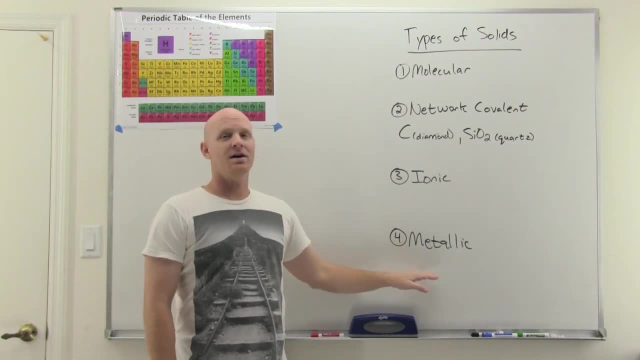 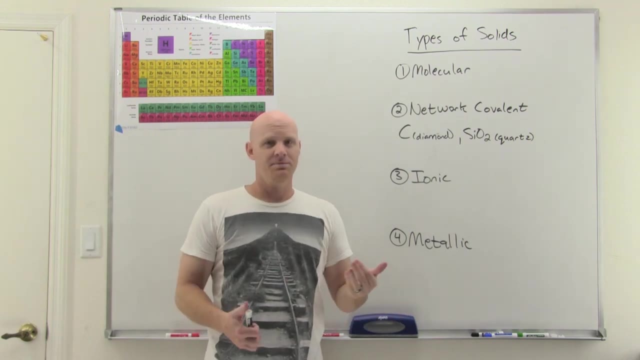 that here again. just wanted to remind you of that. so. but we haven't talked much about metallic compounds and back in chapter eight we talked about them really briefly and said there's kind of this sea of electrons model and we've got these loosely held valence electrons that are 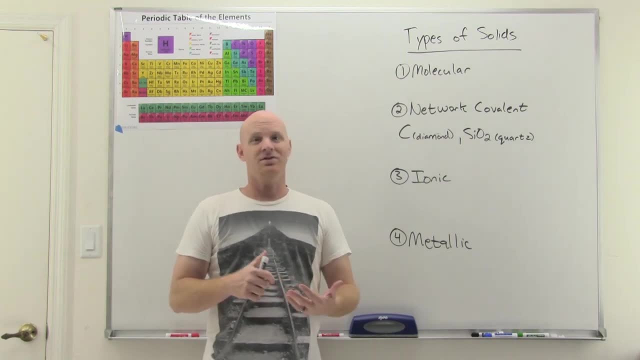 kind of delocalized throughout the whole metal and things of that sort. so we didn't really say much more. but I do want to talk about their melting points for just a second, and so usually the melting is going to be a direct correlation or really, I guess, an indirect. 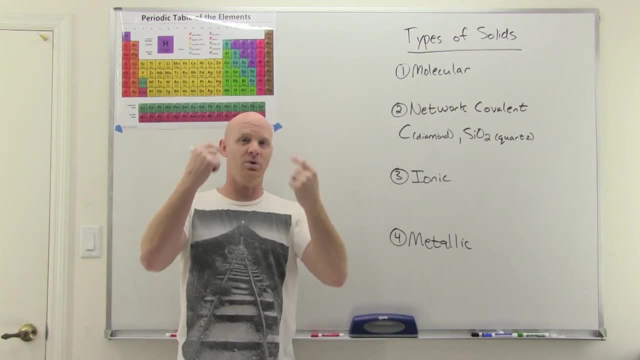 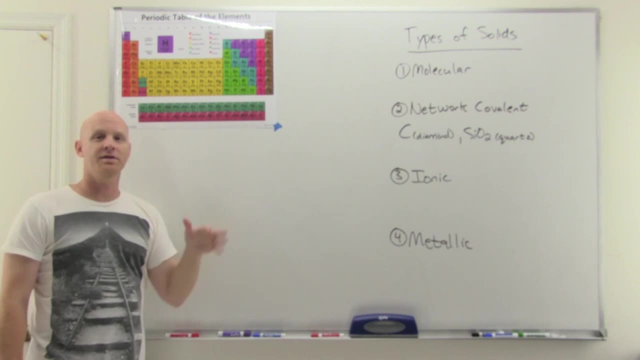 correlation to how strong the bonds are. the stronger the bonds, the higher the melting point. so the weaker the bonds, so the lower the melting point. and so if we take a look at a typical periodic table, so it turns out the strength of the bonding is one related to size, and so 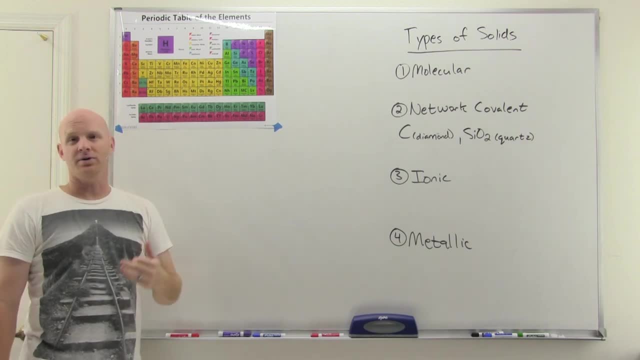 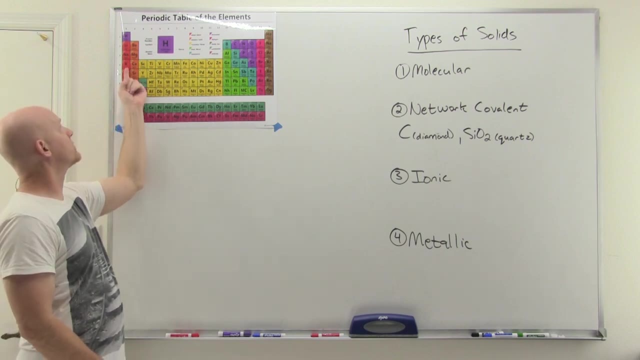 as you go up a group, you get smaller atoms in that metal, and smaller atoms form shorter bonds, and shorter bonds are stronger bonds that are going to correspond to a higher melting point, and so generally, as you go up a group, you get an increase in melting point, whereas 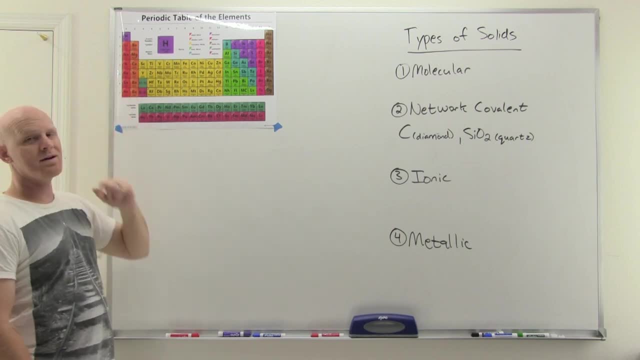 cesium metal here might melt in your hand. by the time you reach sodium up here, I think it's got a melting point somewhere on like 200 or 300 degrees Celsius or something like that. so definitely an increase in melting point as you go up. so the horizontal trend for metals. 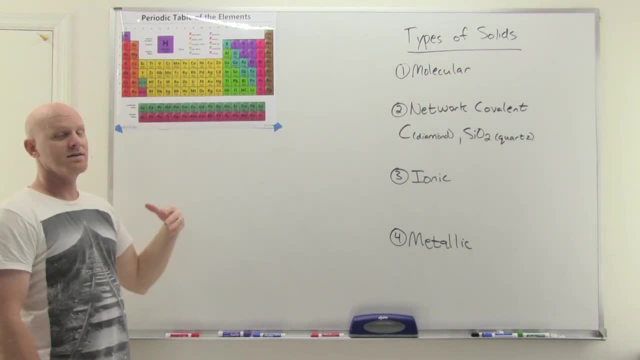 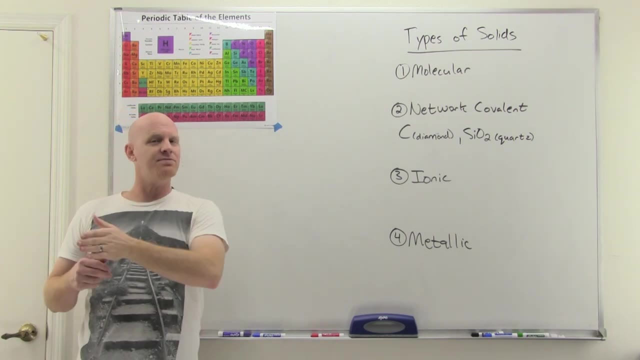 though is a little bit strange, and it turns out, if you look at the horizontal trends, it corresponds well with the number of electrons available for bonding, and you know, usually we think with valence bond theory that half-filled atomic orbitals can be used for bonding.